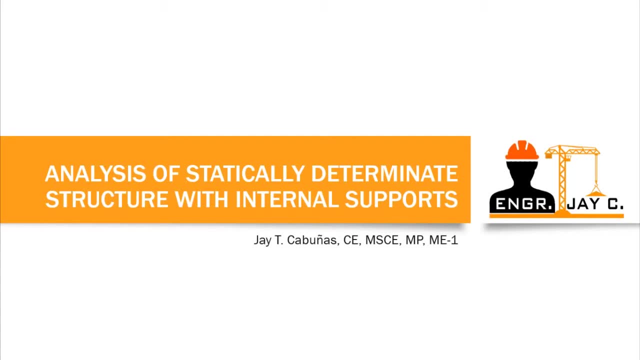 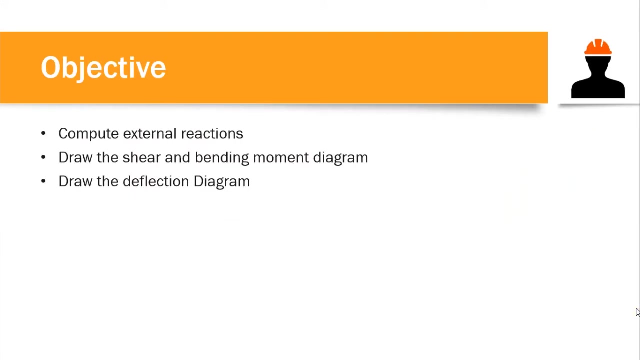 internal ruler and estimating deflection diagram by just looking at the moment diagram. so, unlike with the lesson we had in strength of materials, in which we only dealt with external supports, external loads and so on. okay, so the objective of this lesson is that we will be computing here external reactions, we will draw the shear and bending moment diagram. 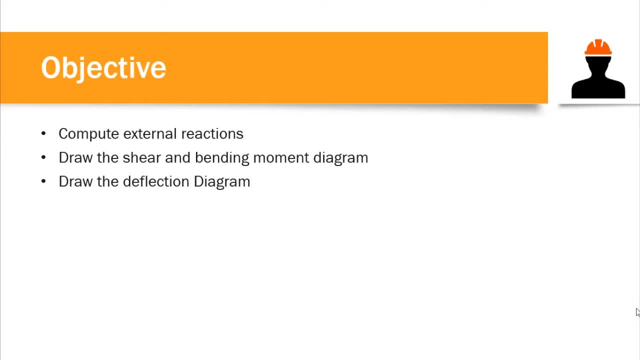 so, the same as with our previous video, and we will also include how to draw or how to exaggerate the deflection of the beam by creating a deflection diagram. okay, so that would be the objectives of this lesson. so let's try to solve an example here. 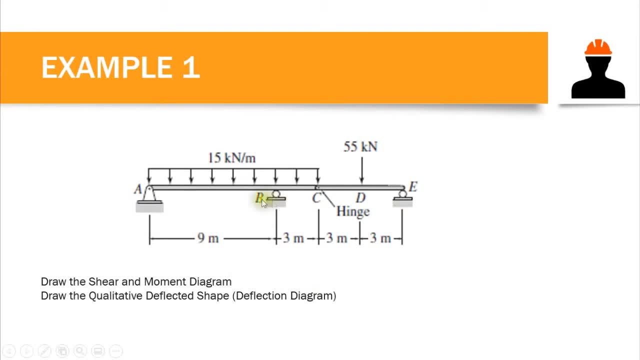 so we have this beam with three supports. so we have um support a, which is hinge support or pin support, and we have b and e here, which has a ruler support. so, upon looking at the beam, we would conclude that this one is an indeterminate structure since, again, we have three support. 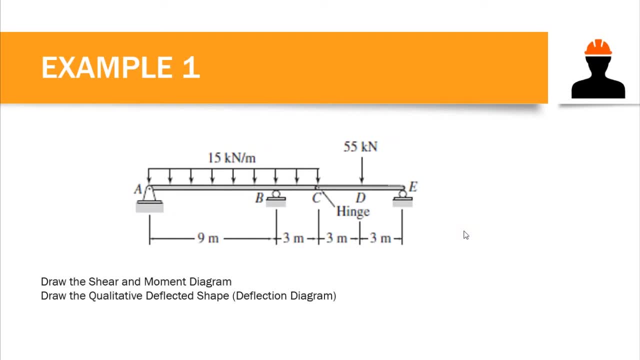 dass. and then we only have: we have four external reactions, but we only have three available equilibrium equation. but take note, we have internal hinge there. this internal hinge makes this entire beam determinate structure. so this is no longer an indeterminate beam, since we have internal supports in this beam. so how are you going to draw the rails? so how do you consider yourve to do all the院? 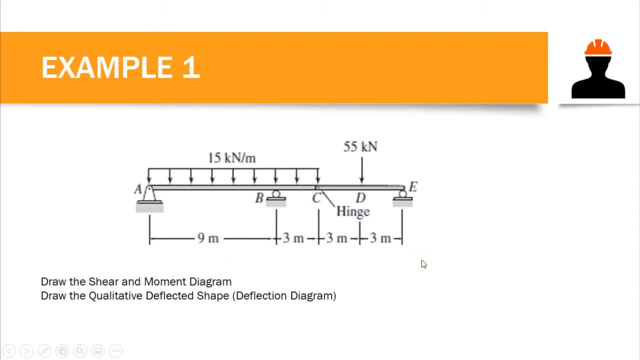 going to check if this one is determinate or indeterminate. so again, we just need to count the number of reactions. so by just following the formula r plus the internal forces, then we compare it to three times the number of rigid. okay, so we count the number of reaction here. so external. 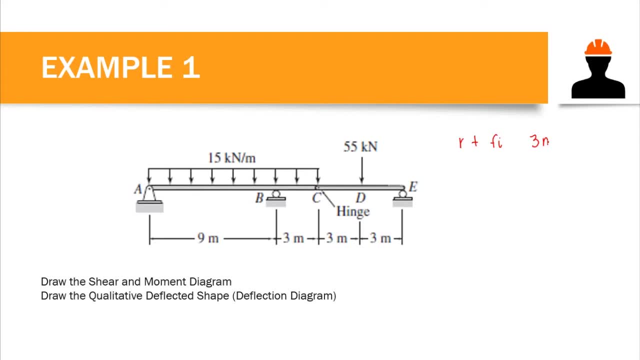 reaction. so since we have um hinge at support a, so we have two reactions, okay, and for a ruler support we have one, and at e we also have one. so for external reactions we have four plus the internal force. so we have internal hinge here and if we cut at this point we would have 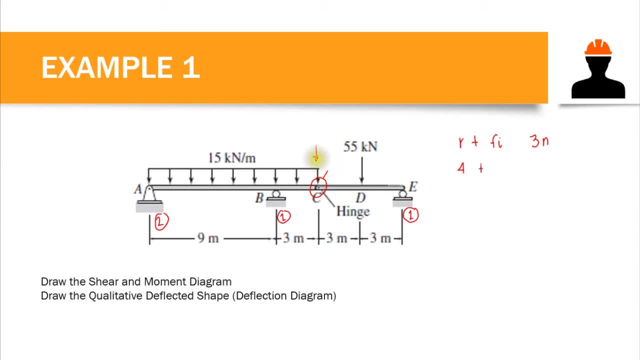 two internal force, and that is um vertical force and horizontal force. so we have two internal forces, so we have six. then for the right side we have three times the number of rigid rigid member, since again we have a member a to c and c to e, so we have a two rigid member. 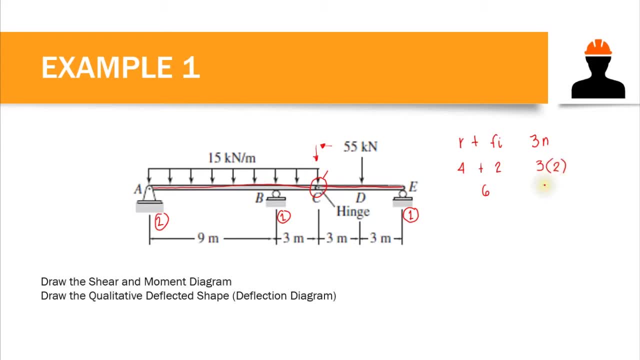 here. so we have two, then three times two, that would give us six. now take note: this right side and left side equations are equal. so that means this one is a determinate structure, or that is statically determinate externally, but for its internal behavior this one is an internally unstable, since we have 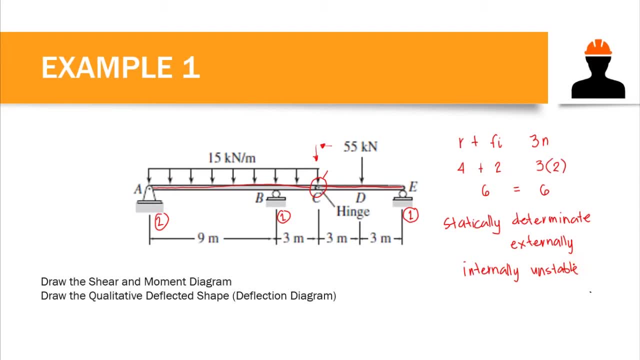 internal hinged in our beam. okay, so the first thing we do here is draw the shear and moment equations. we can use two methods here, by using area method or the shear and moment equations. and then we draw the qualitative deflected shape or the deflection diagram of the beam. 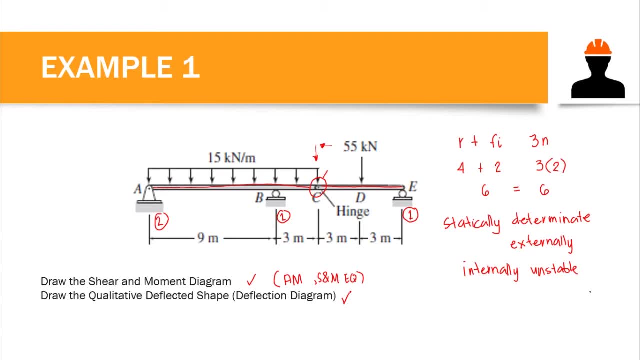 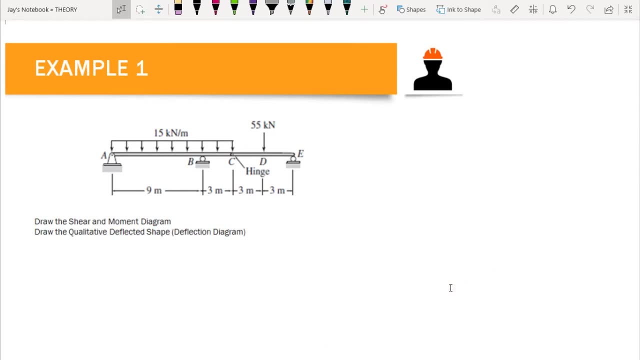 all right, so let's begin the analysis of this beam now, since this beam is a determinate structure, so we will be using the equilibrium equations in computing its external reactions, or external forces. okay, so those equilibrium equations, such as summation of forces vertically, summation of forces horizontally and 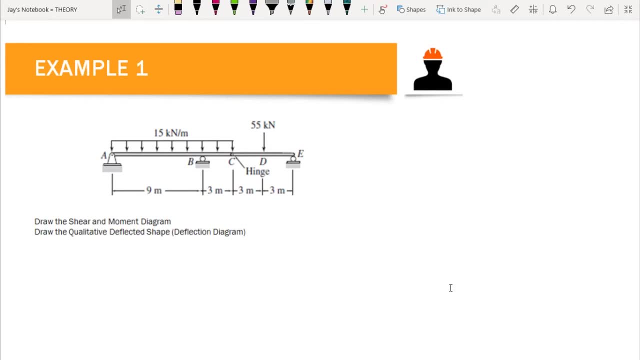 summation of moments are enough in computing the external reactions. however, since we have three supports here with four external reactions, so we will be um cutting this beam into two. okay, so we will be cutting this beam at point c, which is the location of our internal hinge. 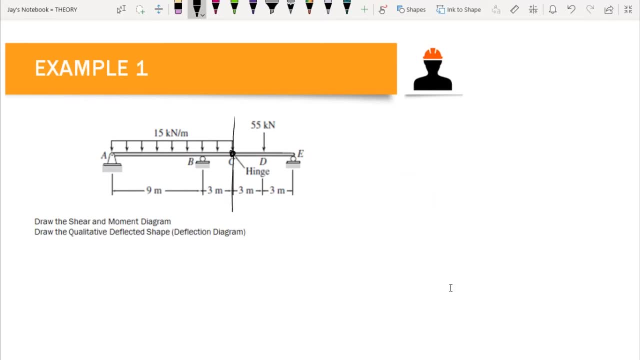 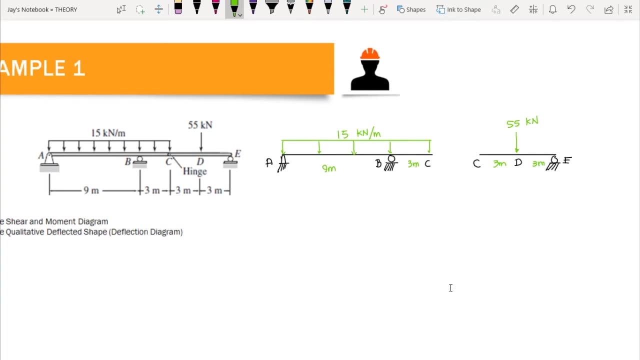 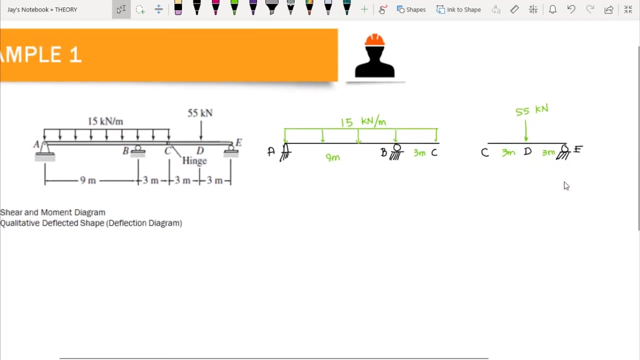 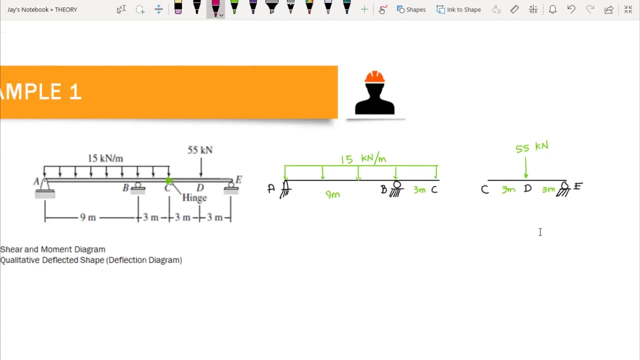 so we will be cutting at this point here. so we have a two segment here. so we have a segment abc, so we have a segment abc and c, d, e. okay, since again we have two rigid members here. okay, now at point c, since point c here is internal hinge. so therefore we only have two internal reactions. so 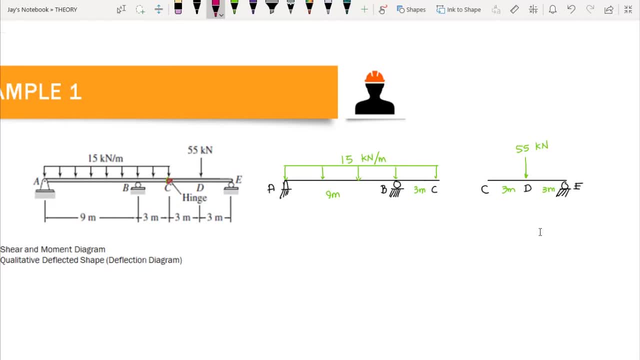 we have um forces vertical and force horizontal, okay. so we do not have moment at that point there. so we have a, let's say that is, we have cy that goes up and we have cx that goes to the left, okay, and on the right beam or the right segment, so we have the same magnitude. 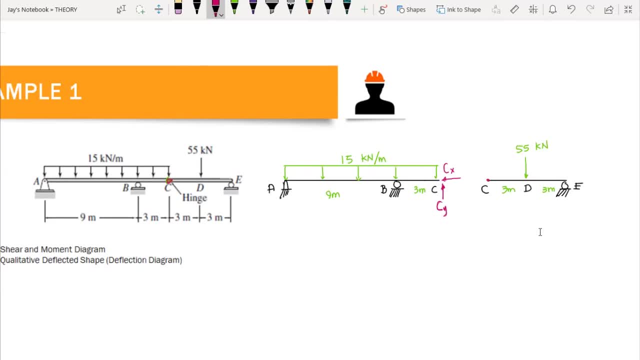 but opposite in direction. okay so, since on the left side of point c we have upward vertical force. so therefore on the right side we have a downward internal force- let's see why- and a rightward horizontal force. that is our horizontal force cx. so again, they have opposite indirection, but they always have the same magnitude. okay, now at 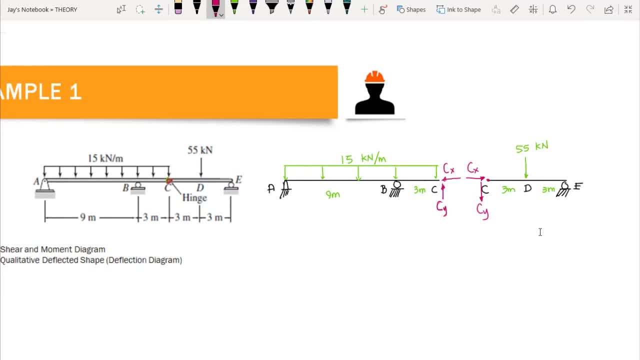 point a, since this one is a hinge. so we have two reactions. we have vertical, let's say it's ay and ax. now at b, since this one is a roller support. so this mean this: have only vertical reaction. that is by and for the support at e, since, again, this one is a roller support. that means this: 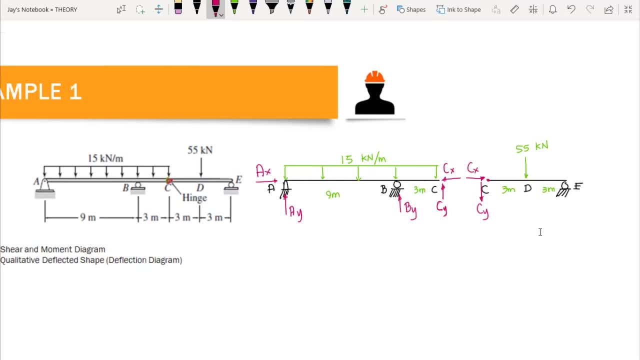 only have one external reaction and that goes upward, or so let's assume that this one is upward force. that is ey okay, so we can now compute, or we can now determine the reactions. okay, by first computing reactions. e okay, since we cut this into two segments, so we will be analyzing the two segments individually. 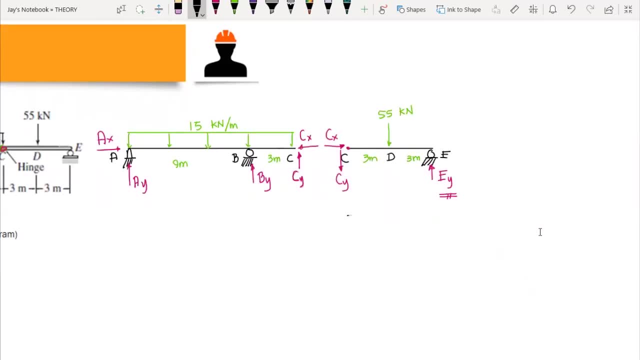 okay. so we sum up moment at C and this one is equal to zero. so we assume that all the force is rotating counterclockwise are positive. so if we sum up moment at C, then we only have two forces that would be included here or two forces that would be included here. so if we sum up moment at C, then we only have two forces that would be included here or two forces. 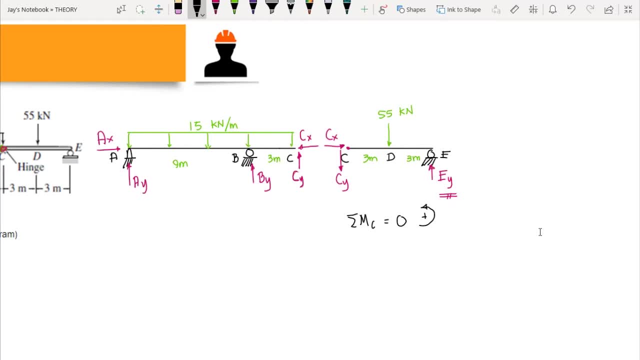 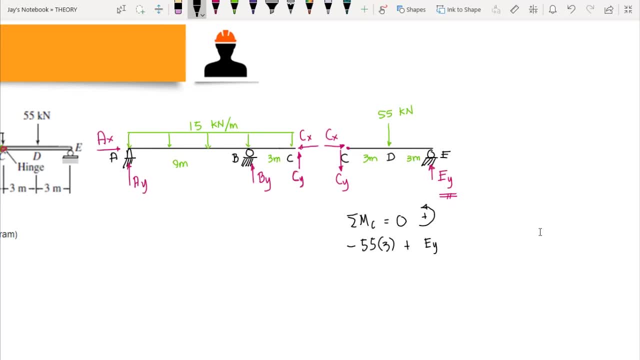 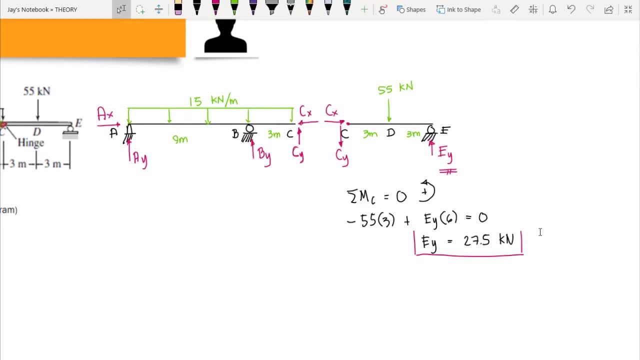 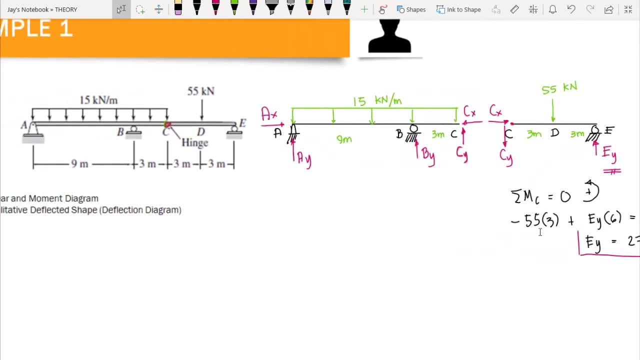 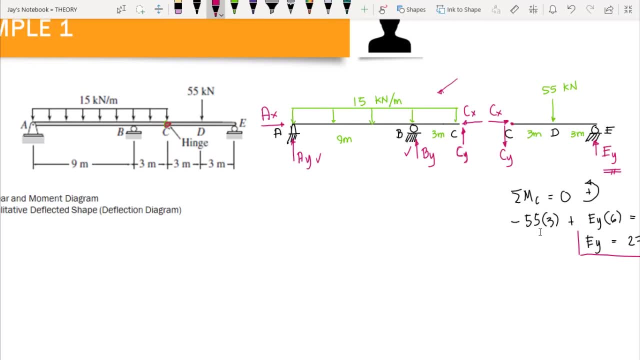 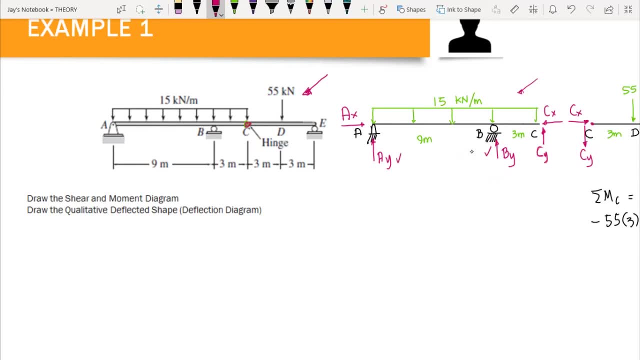 um, analyze these beams individually now. okay, so we will analyze this beam as a whole now. okay, now take note, we have the value of our ey here, which is 27.5. okay, and that goes up since we have positive value. so we have again. we have ay here and ax. 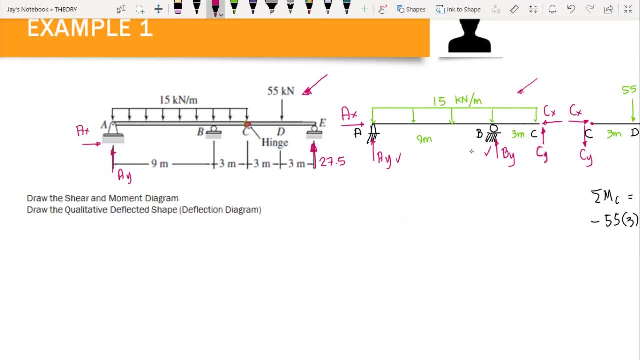 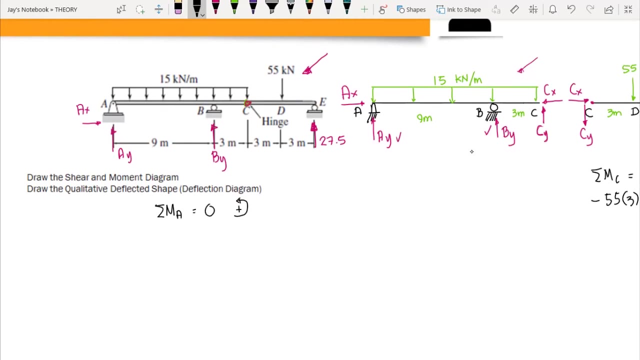 we also have by here, so we can compute by here first, by summing up moment at a. okay, so we sum up: moment at a is equal to zero. so all the force that rotates counterclockwise are positive. so we have 27.5. so this one is positive. since this is counterclockwise times, the moment arm of 27.5. 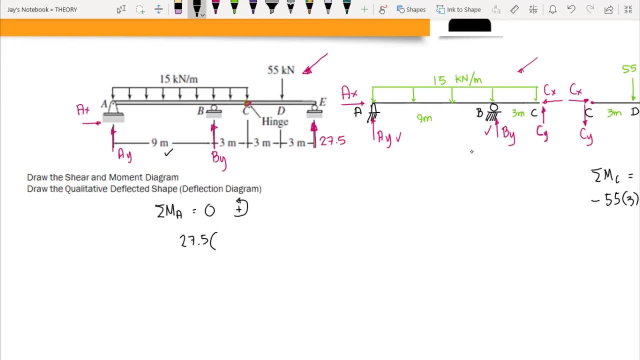 from a. so we have 27.5. so we have 27.5, we have nine plus um. this one is nine as well, so we have 18 meters. okay, the perpendicular distance of 27.5 from point a. then we have by. so again, this one is b. this one is positive, correct, since 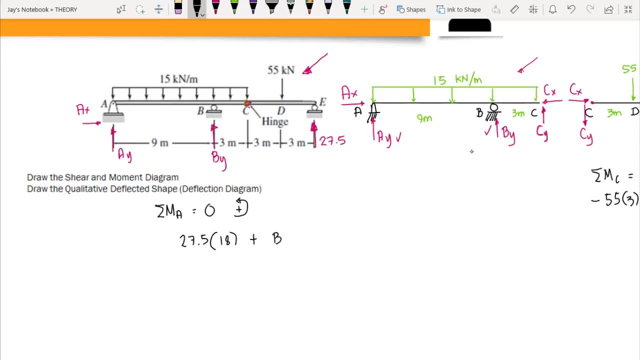 this rotates counterclockwise, so by times the moment arm from a is nine meters, so we have nine. now, take note, we have external load, so we have uniformly distributed load here. the resultant of this one is 15 times. now. our uniform load here runs from 0 to 12, correct? so this one is 12, since 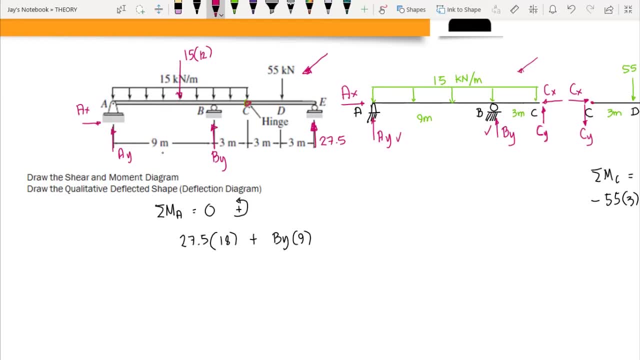 the length of our uniformly distributed load here is 12. we have 9 plus 3 meters. okay, then 6 meters is the. the moment arm is six meter. that is the location of our resultant the distance from point 8 to the center of our Uniformly distributed load. okay, since again we have 12. 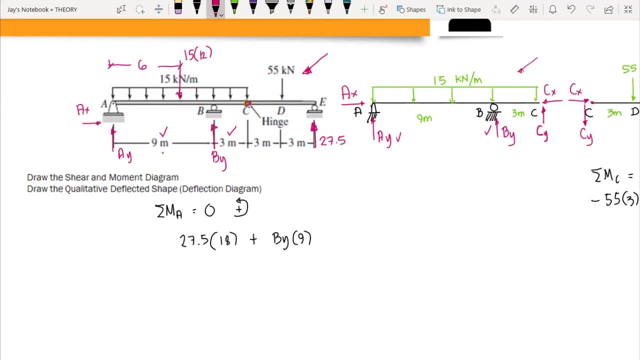 meter as the length of our uniformly distributed load. so we have here 15, that is, uniformly distributed load times 12.. This is the area of our load times, the moment, arm 6. Now the rotation is clockwise from point A. that means we have negative. here. We have external point load which is 55 kN. Now 55 kN location is at point D, which is 15 meters from point A, Since this one is 6 meters, it's correct. 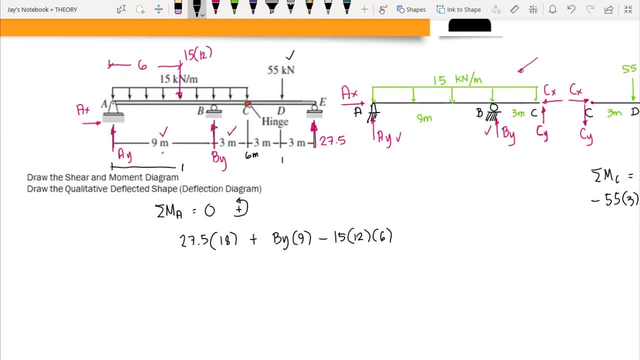 So from point A we have 15 meters distance, So we have 55 times 15.. The rotation is counterclockwise. that means this one is negative, Then this always equates to 0.. Okay, so we can now compute By here, and By here equals to 156.667. 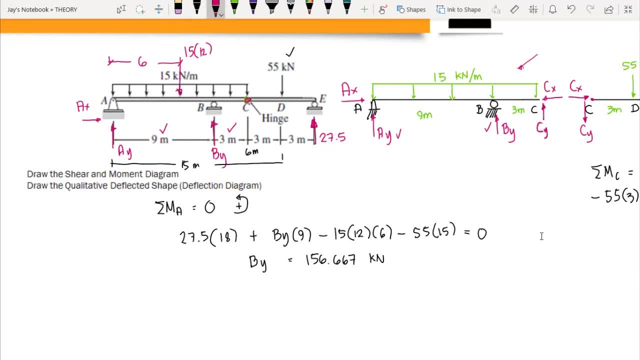 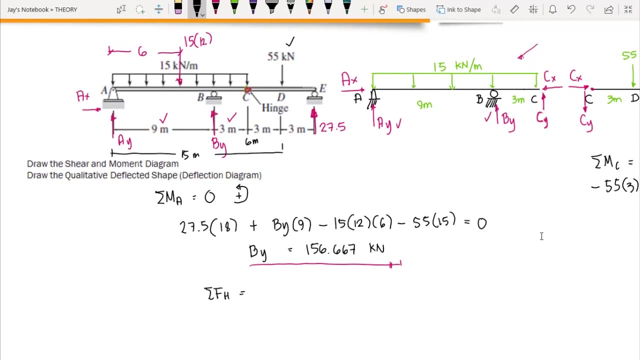 So we have now the reaction at B, So we only have remaining reaction here, which is the reactions at point A. So if we sum up forces horizontally, so we have summation of force horizontal is equal to 0. Again, this applies to the entire beam. 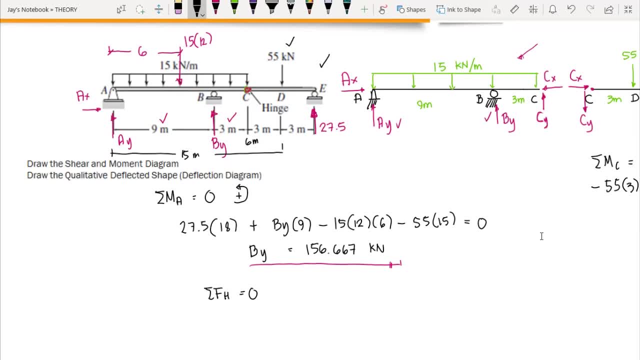 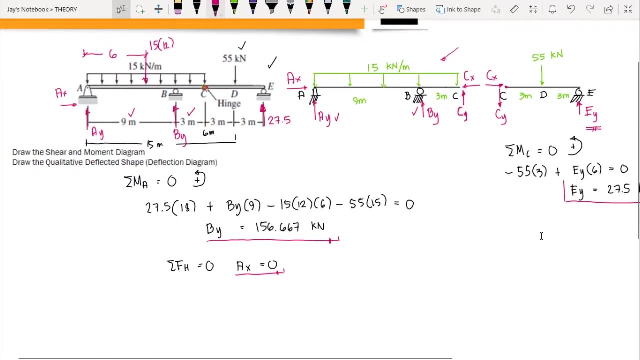 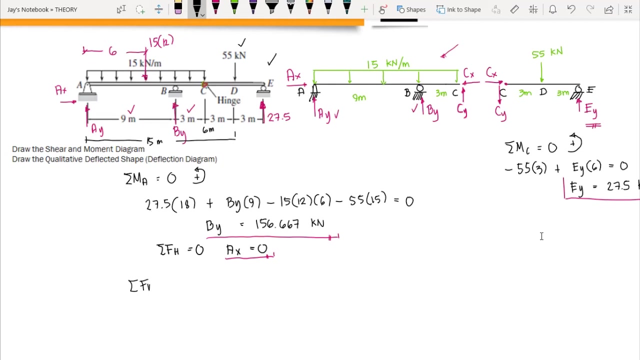 So we only have one. we do not have external load that acts horizontally correct. So that means we can say then that 1 reaction at A or horizontal reaction at A is equal to 0.. How about the vertical reaction at A? So we can sum up forces vertically? So we have summation of forces: vertical is equal to 0.. Upward forces are positive. 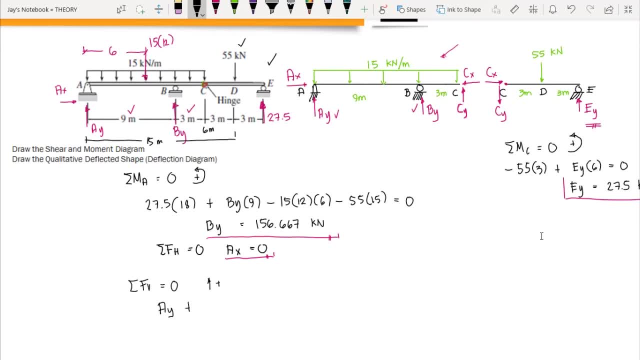 Then we have Ay plus By, plus Ey, minus the resultant of the uniformity distribution. So we haveと제,6 15 times 12 minus 55 is equal to 0. So we have Ay plus By. we have already computed the value of By here, which is 156.667 plus Ey. 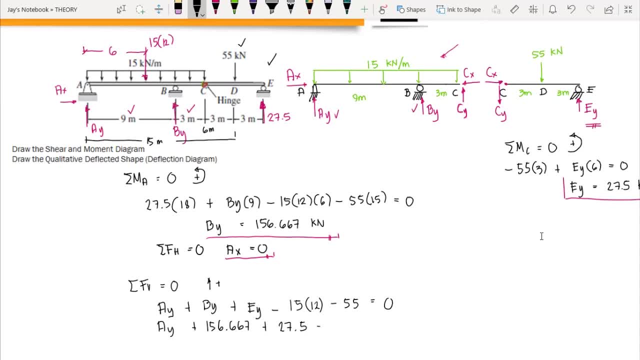 Ey is 27.5 minus 15 times 12 minus 55 is equal to 0.. So this is theningונected value. So now let's compareзе: find円, then Other, and and the beck is transgendered. 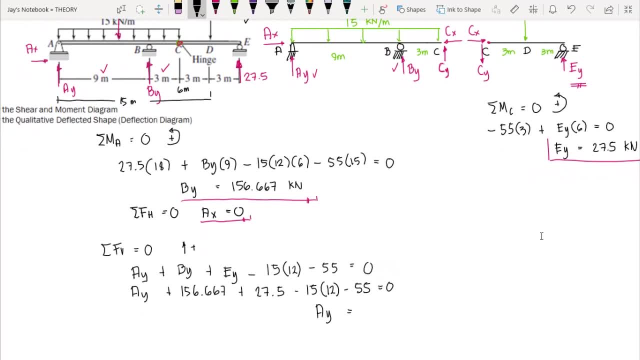 this would give us the value of our ay, which is equal to 50.833 kilo newton, and this is acting upward. okay, by is acting upward as well, and the same as with ey. so this is our reaction at ay. so this is how you compute reactions for beam with internal hinges. again, this is not a simply supported 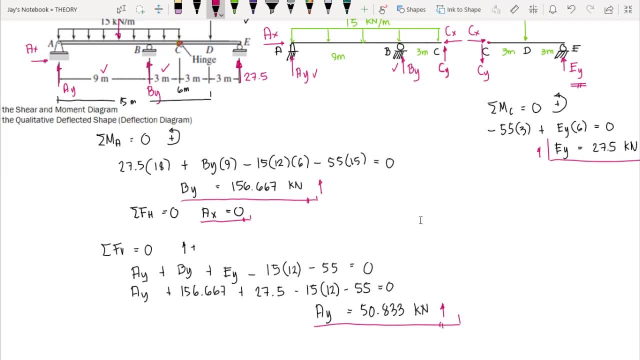 beam again in simply supported beam. we have only two supports, that is, hinge and tooler. but take note, here we have three supports and with one internal supports. okay, so you just cut the beam into two or more segments based on the number of rigid members. okay, so then our goal here is to 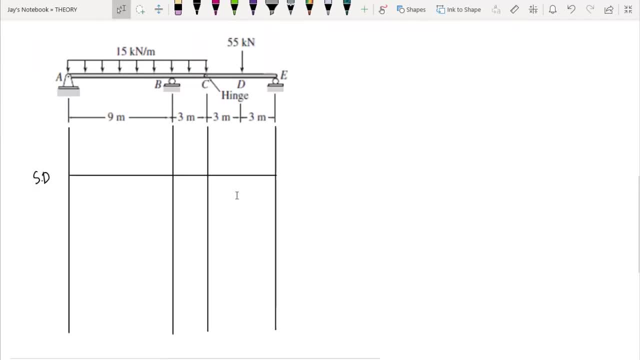 draw the shear and moment diagram. so in creating a shear and moment diagram, so we have two approaches. so first we have area method and the shear and moment equation method. but the easiest and the simplest one is by using the area method. so if you have not watched my 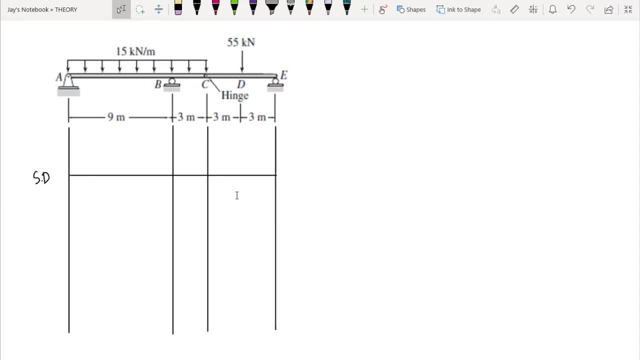 video regarding these two methods in creating a shear and moment diagram. please watch my previous discussions on these lessons. i have posted the link in the description. so let's now draw the shear. and now let's try to draw the shear diagram first. now we have to write first the reaction. so for at support, a ey is equal to 50.833 kilo newton. for b by here is: 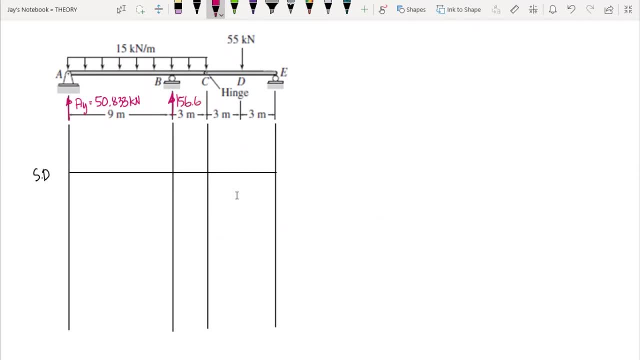 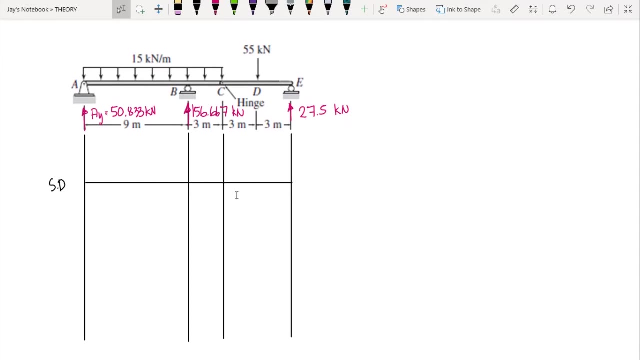 equal to 156.667 and 50.833 kilo. newton for b by here is equal to 156.667 and 50.833 kilo. newton for b by here is equal to 156.667, and at support e the reaction is 27.5 kilo newton. so let's begin at the leftmost support, which is: 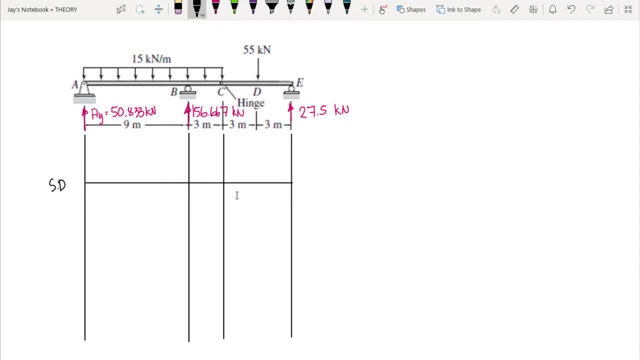 point a. so at leftmost support, our initial shear there is is 50.833. okay, so we go up at point a, since ay here is acting upward. so our point here is on the top of our datum, which is this one. this is our datum zero. so we have 50.833 there. then now take 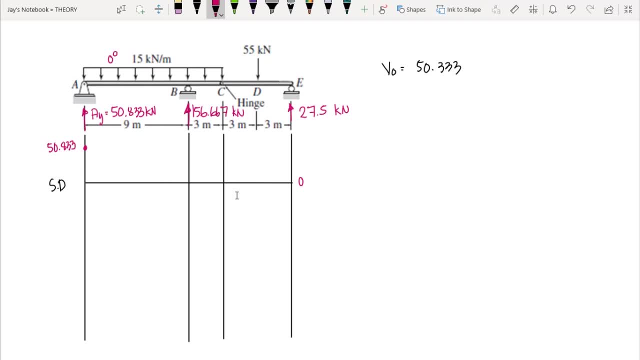 note: this is in zero degree, our load is in zero degree, so therefore our shear diagram should be on the first degree order or on the linear equation or linear graph. so we have our shear one. okay is equal to 50.833, okay, minus the area of our load, which is 15 times nine. so this gives us negative. 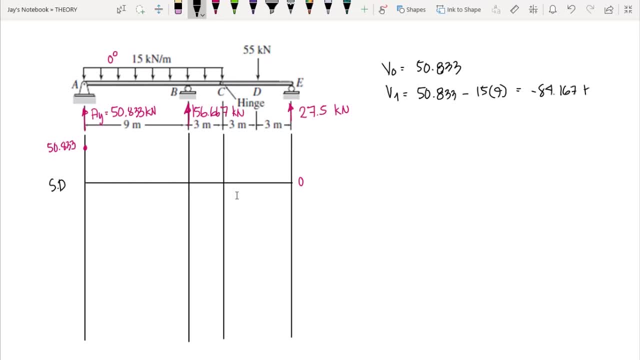 eighty four point one, six, seven kilo newton, since this one is negative. so we plot our points below the datum or the reference line. so we have at this point here let's say this one is okay at this point. okay now at support b or a point b. we have know that at support b, point b swing. 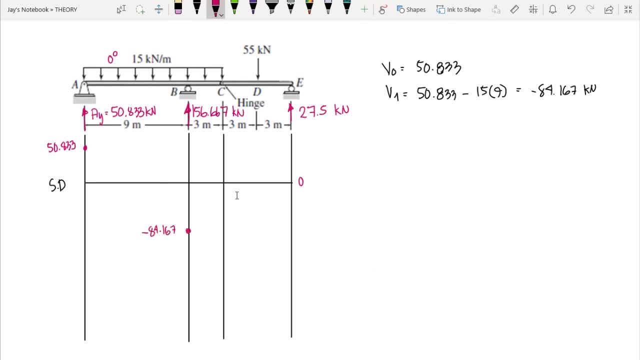 is negative eighty four, point one, six, seven, so this here is one, so we connect the two points, so we have this one. okay, now at support b, or at point b, we have upward reaction which is 156.667, so we have second: here is negative 84.167 plus 156.667, so this one here is. 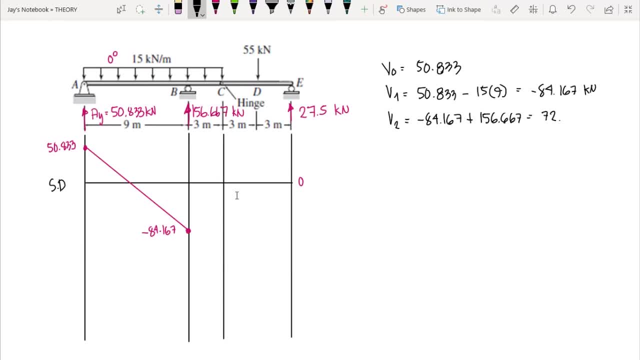 this equals to 72.5. okay, so we go up, so our point is 72.5. so let's say at that point, so we have 72.5. okay, then at that point, at our point c, so let's say: that's our third shear force, so is. 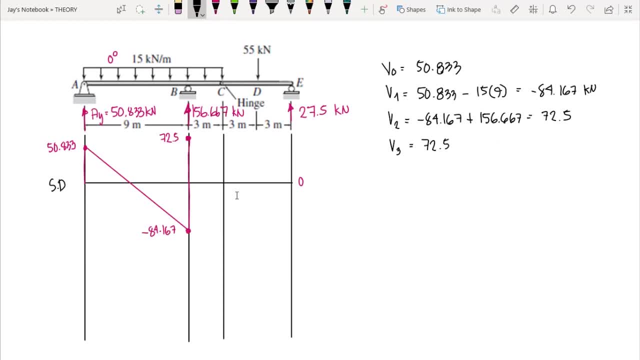 equal to 72.5, since our uniformly distributed load here is going downward. so this one is negative. 15 times 3, that is the area of our load above bc. so this equals to 27.5. so we have to move downward. so at this point that's positive, so we have 27.5. then we connect the points. 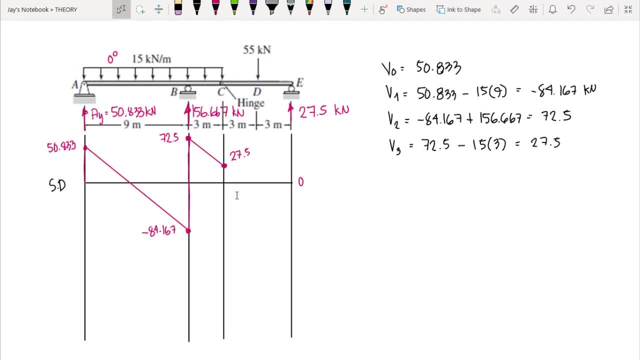 and this 27.5 here. this is the value of the internal force cy. okay then, at that point- now take note- we do not have a load from c to d, so we have a zero degree at that point, so we have a horizontal line at this point. okay then, since we have a, so our v4. 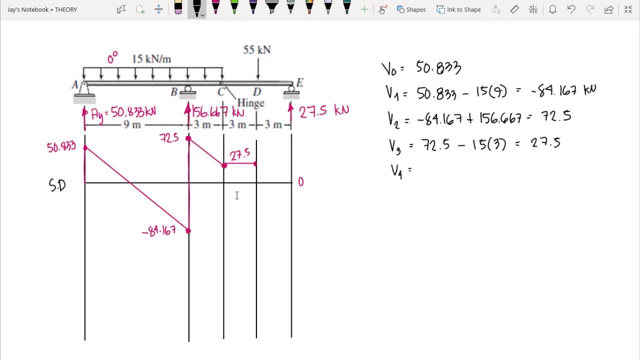 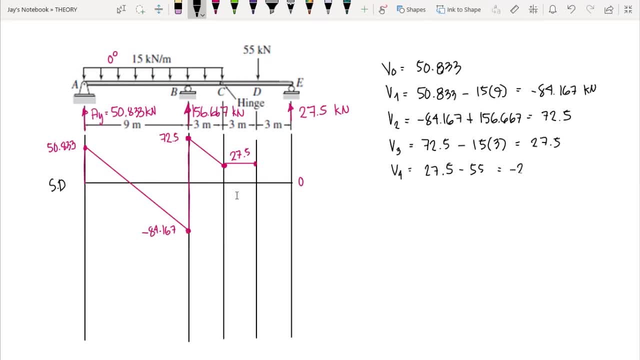 and this equals to negative 27.5. so we have um at this point. okay, so we go downward, so we have negative 27.5. now we do not have load between d and e, so that means we have zero degree line. so we have this line. now take to that point e, we have 27.5 reaction, which is going. 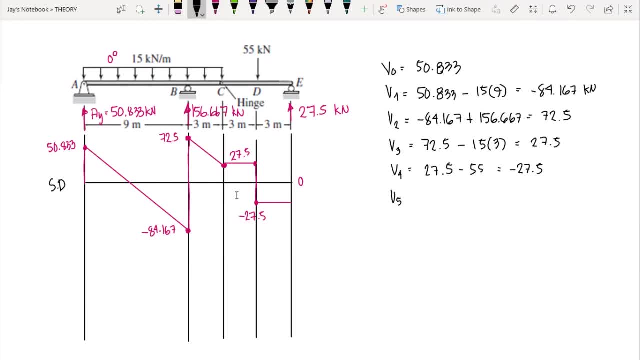 upward, so at v5 of our, our final shear. so we have a negative 27.5 plus 27.5. this gives us zero. so that means, since we end at zero shear, so that means we have correct shear diagram. so we have correct shear diagram again, since we have our final shear equals to zero. so this one 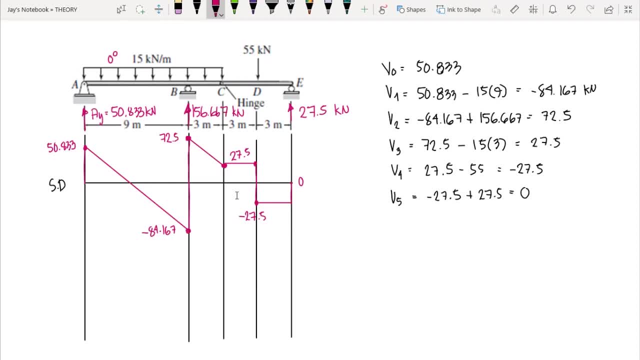 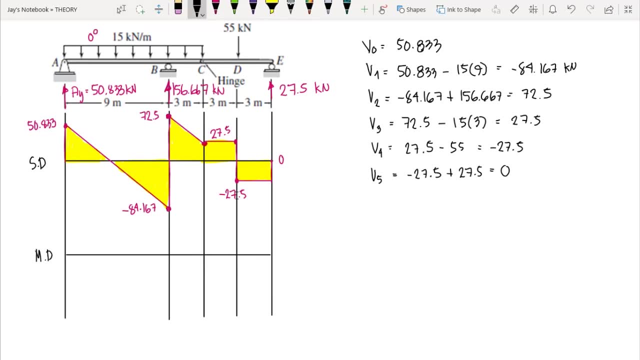 now is our shear diagram for this beam, and now let's draw the moment diagram. so we will still be using the area method. okay, the simplest and easiest way in drawing the shear and moment diagram. so now let's proceed. or let's start from the left, most of our beam, which is at point a now, since, again, this is a hinge. so therefore we do not have 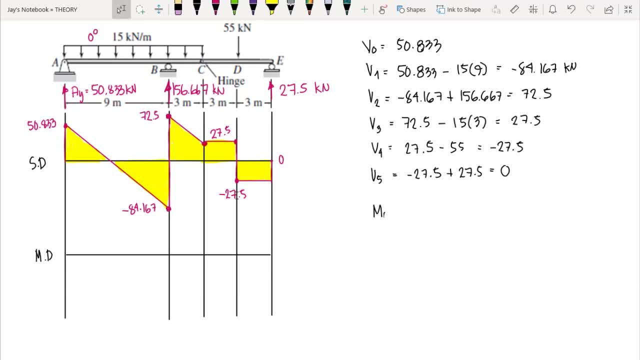 moment at that point. so we start at moment zero, or that is zero kilo newton meter, okay. so that means at that point we have zero moment. so and then we proceed. at this point let's say that is our point, a prime, okay. now, at this point we have zero shear, okay. 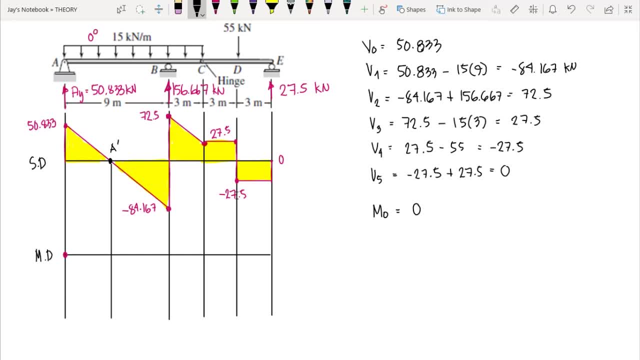 that means from, since we have a zero shear there, that means that is the location of the maximum or the highest point of our curve. again, the location of the highest point of our curve is where our shear becomes zero. okay, so at that point we have the maximum point of our parabola, or our second. 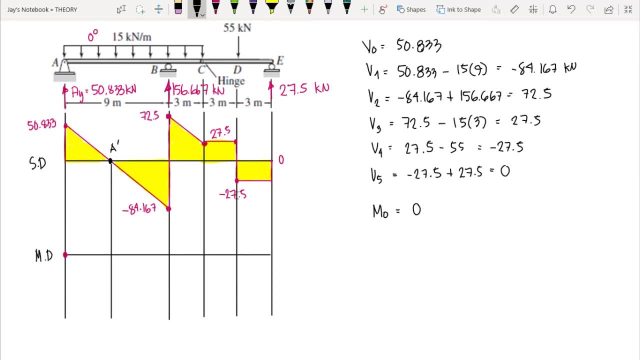 degree curve. okay, so how are we going to compute? so we have um the area of the shear diagram above this point. okay, that means we have. however, we do not have the um the distance, since this one is a triangle and we will be needing the length of its base. okay, so how are 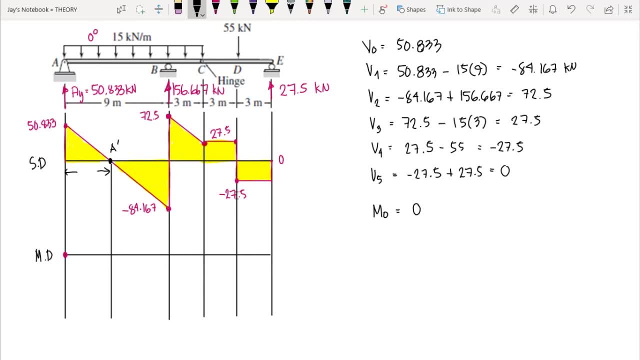 we going to compute that length there so we can use the ratio and proportion. so by ratio and proportions we have 50 point eight. three three is two. let's say that's x. okay, over x equals to 84.167 over. since we have nine meter as a total length from a to b, that means this length here is nine minus x, correct, okay? 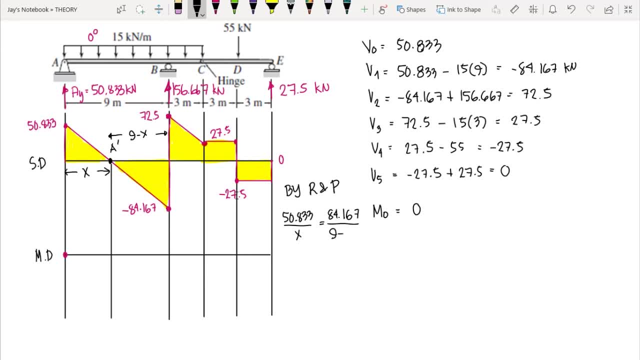 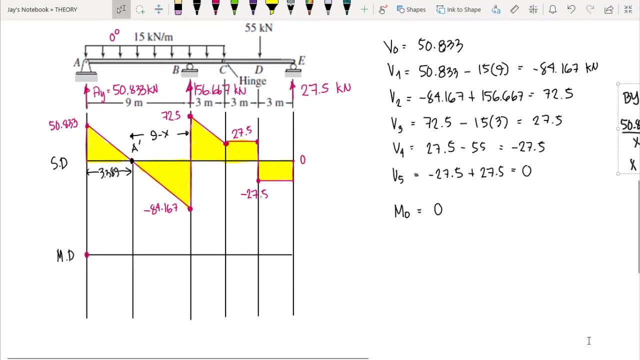 that's nine minus x, so we have over nine minus x. so by um, evaluating it further, we have: x is equal to. so you can use your algebra, or if you have your calculator then you can directly compute it by shift solve. so we have the value of x, which is 3.389 meters. so we have a 3.389 as the distance. 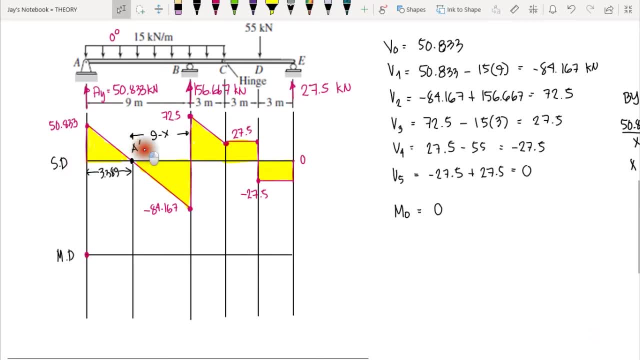 from point a to a prime. therefore, from a prime to b, we have 9 minus x. that would give us 5.611, okay, 611 meters. that is the length from a prime to b. so we can now compute the area of the shear diagram. so let's say that's our m1. this equals to we start at zero. then that's positive, since that is a. 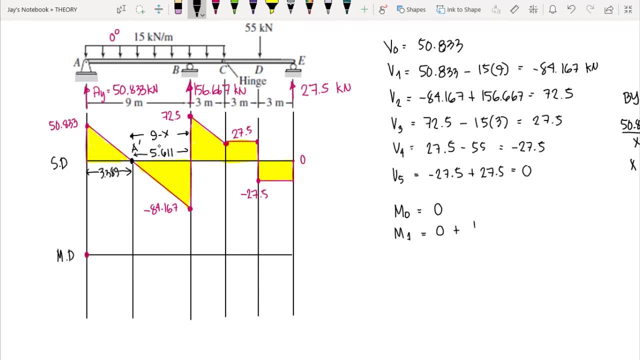 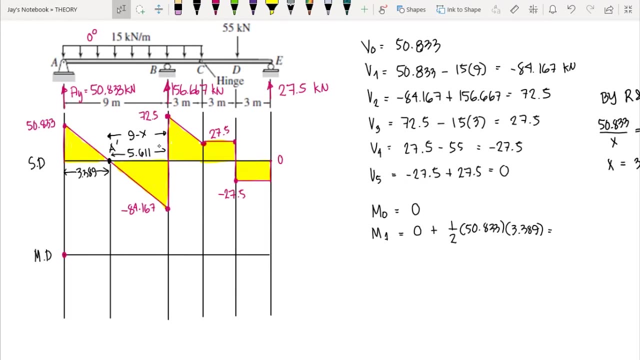 positive shear area, that is, the area of a triangle. one half 50.833 times the length of our triangle, which is 3.380, gives us our moment one: 86.137. okay, that's positive moment. okay, that is, let's say, at this point we have 86.137. okay, now that that is the highest point of our curve, since, again, that is, 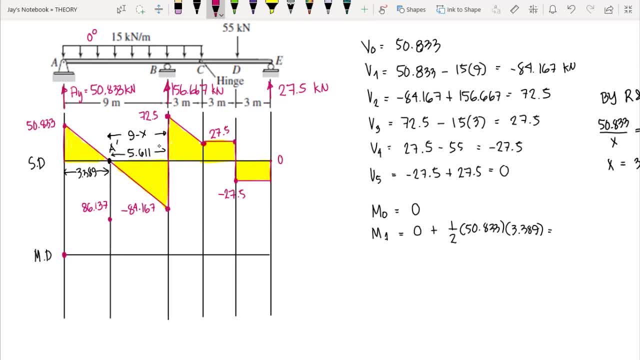 the location of our zero shear. so we have a second degree curve. now this one is concave downward, since we have a decreasing magnitude of our shear diagram. okay, since we have decreasing shear force. so that means we have a frowning curvature, okay. so if you are not familiar with the orientation, 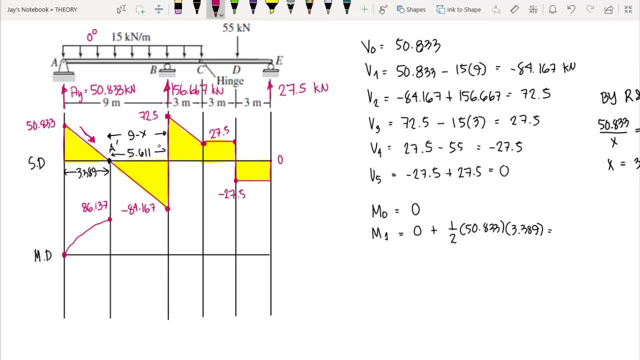 so i have posted a discussion on how to draw the shear and moment diagram on the description below. okay, so let's proceed to the second moment. so we have now- let's start with- positive- 86.137. then we have negative shear area, which is negative one half times the area of this triangle, this one, which is 84.167. 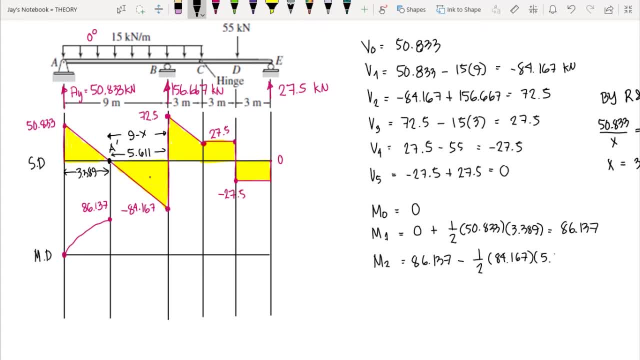 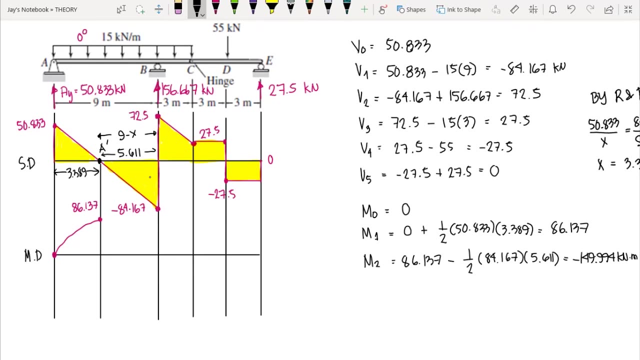 which is the area of this triangle, which is 86.137 times the length of the triangle, which is 5.611.. This would give us negative 149.994.. And this one is kilonewton meter. So we have negative 149.994, which is below the reference line. 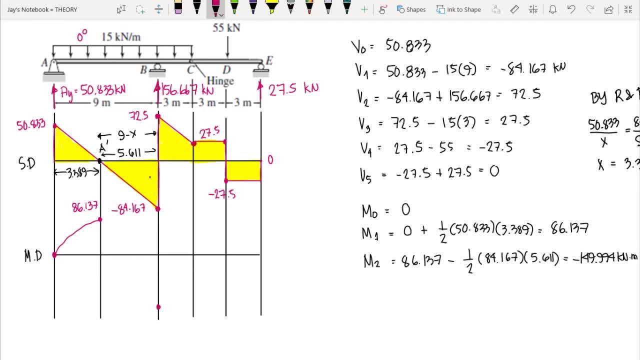 So we have at this point here- Let's say that is negative- 149.994.. And since this is also a going downward force, that means we have a frowning curvature, And that is in second order, since this one is first order. 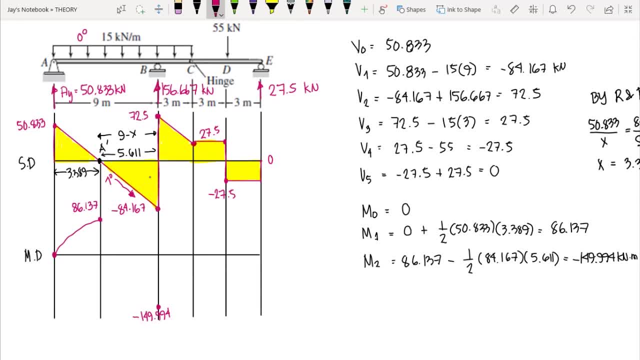 So the moment diagram should be on the second order. So that means we have parabolic curvature. So this would be, This would be our curve, which is a parabolic curve. Then we proceed to moment 3.. So at this point here, 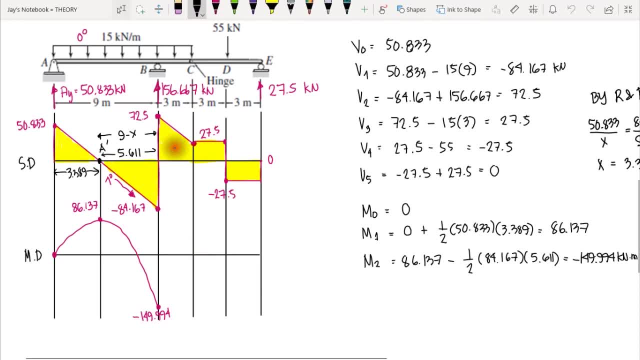 Now take note. we have the area of our trapezoid, So we have moment 3.. We start at negative 149.994.. Then positive area. Since that area there, this area is above the reference point, Or that is positive area. 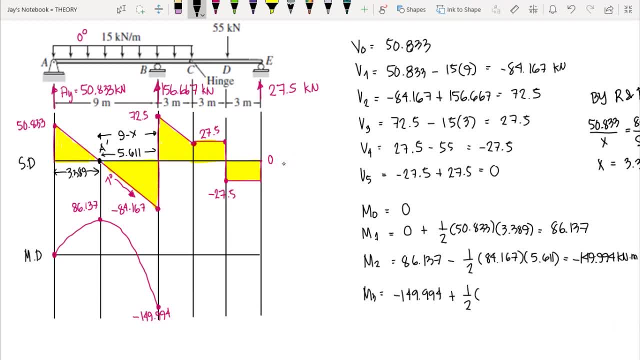 Now we have the area of the trapezoid, One half times 72.5, plus 27.5 times the length, which is 3 meters. Okay, This one So times 3.. This would give us 0.. 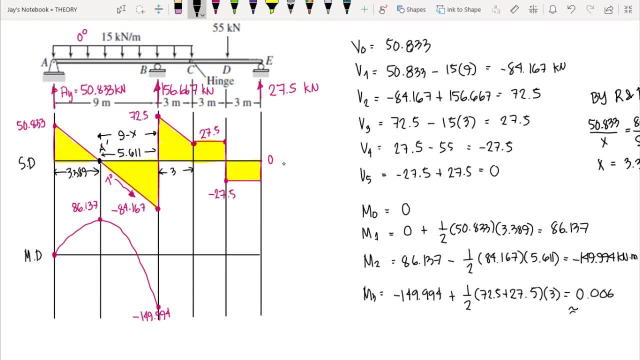 Okay, Or 0.006.. So this is approximately equal to 0.. Why 0?? Now take note at point C: this one is internal hinge, Correct, Correct? So at point C, c, we should not have internal moment, since that is a hinge. so we have only two internal forces. 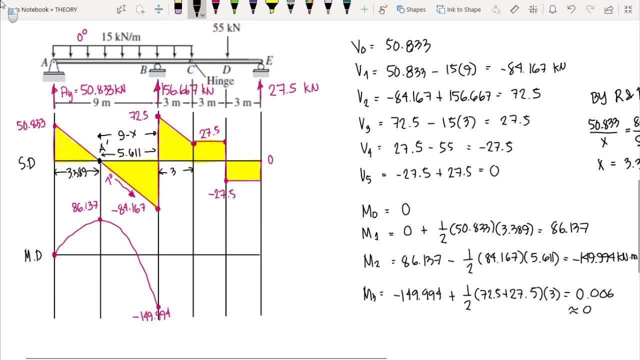 that is the vertical and horizontal internal force. so no internal moment. so that would justify why we have zero moment at c. okay, now we have the curvature, which is frowning curvature or concave downward, since we have a downward shear force here. so that means we have this. 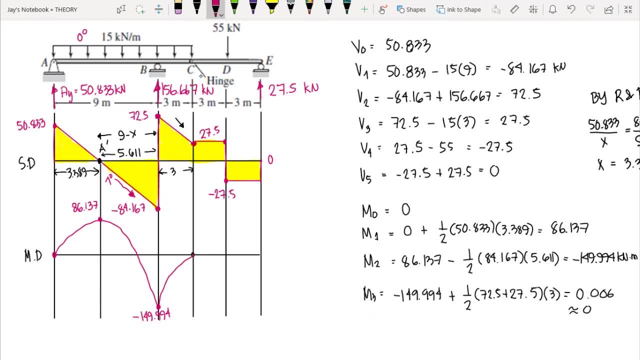 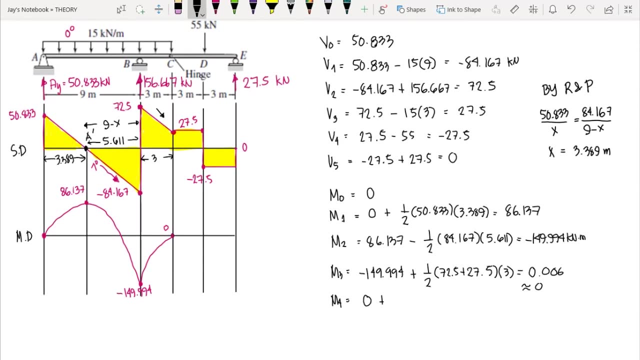 curve. okay, so we stop at zero now, at c to d. so we have moment four. so we begin with zero moment. plus the area of our shear diagram, this one, so we have 27.5 times 27.5 times c to the power of c. so we have moment four. so we begin with zero moment. 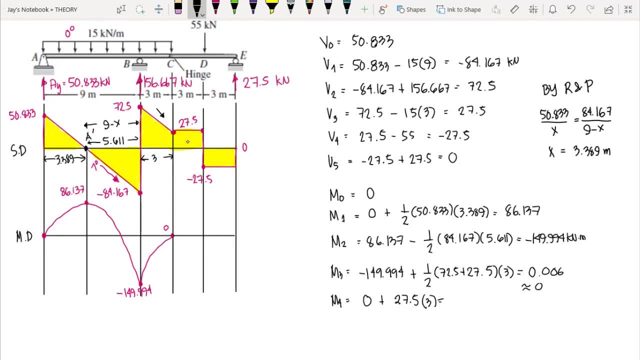 three. this would give us 82.5 kilonewton meters. so this is the moment at point d. now take note: this one is zero degree order. that means we have a linear or a line graph here. okay, so we have first degree moment diagram, so we have 82.5. so at this point let's say, at that point 82.5. 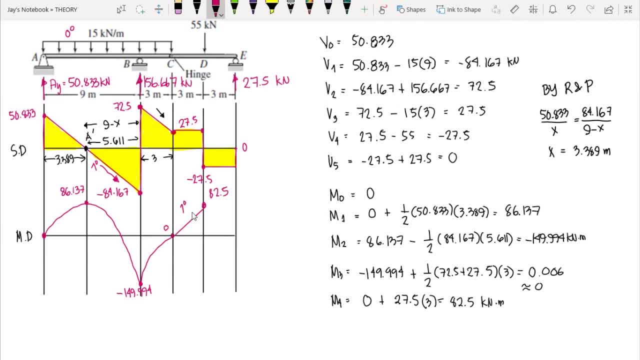 okay, so we have a linear or a line graph here. okay, so we have a linear or a line graph here. um, so we have a investigate, So we have a first degree moment diagram and then, um, at our final moment, so we have M4. so we begin with 82.5 moment, then minus the negative area, since this camera is making thatамен. 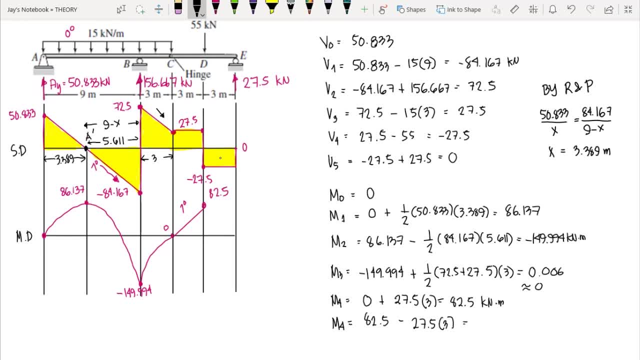 negative shear area, so we have 27.5 times three. this would give us zero. so that means we have 고 negative shear area. so we have 27.5 times 3. this would give us zero. so that means we have course m虹, which is 8, d work as an yelling nu pharmacy model. so we have rhyme, and this is the point you can review. 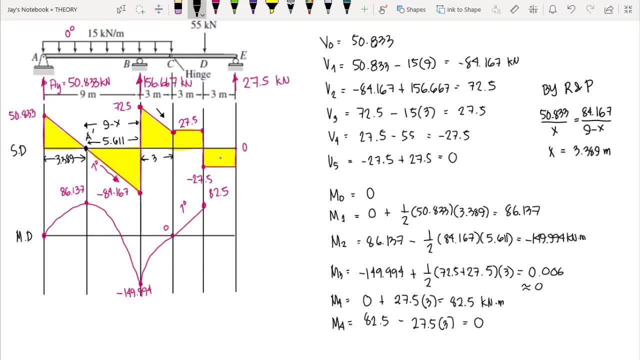 we have correct moment diagram, since we end with zero moment diagram. so we have on this moment diagram for our beam. okay, so you can try to draw the shear and moment diagram by using the shear and moment equations. so we are done with shear and moment diagram. now let's try to draw the 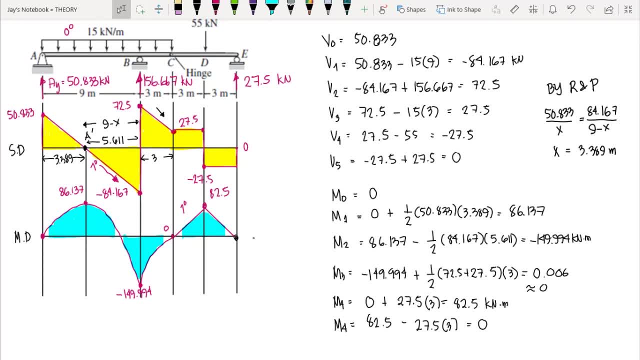 deflection diagram. okay, so let's exaggerate the deflection, since in reality, the deflection should be small, okay, that is, in millimeter or so on, but for this one, in order to internalize the behavior of our beam, so we would try to draw the deflection exaggeratedly. okay, so, in drawing the deflection, 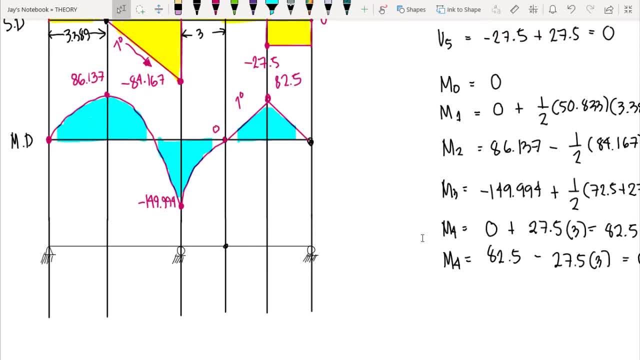 diagram. we will just be needing the moment diagram. okay, so we will just try to look at the moment diagram. so if we have a positive moment diagram, that means we have a smiling bending diagram, correct, since we have smiling face. now. for a negative moment, that means we 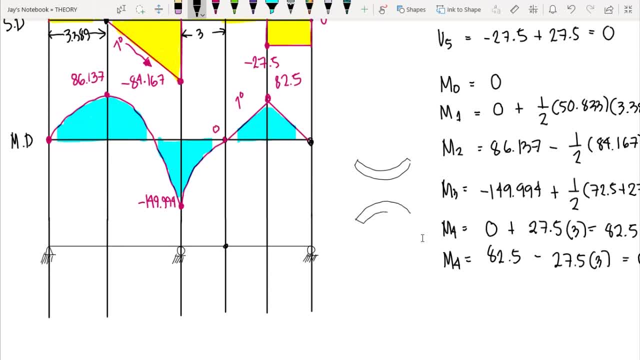 have a frowning bending, okay, that is a frowning curvature for deflection diagram. now, at the point where we have a zero moment, okay, that is the point of inflection, okay, inflection point. inflection point is where our, where the curvature of our bending diagram. 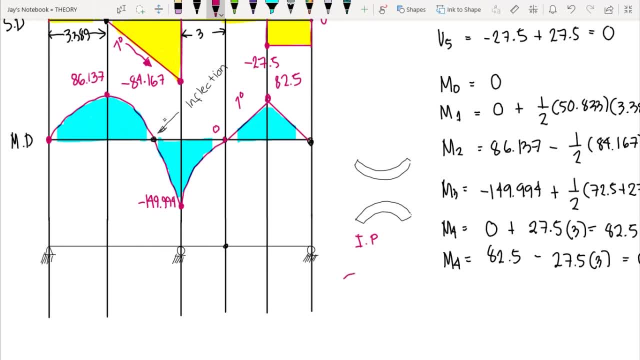 changes, like it changed from a concave downward to concave upward, okay, from frowning to smiling curvature. so at that point- this is what we call the inflection point- okay, or where our beam changes in curvature, okay. so let's start with at point a or at a. now take note, this is a hinge, so that means we do not. 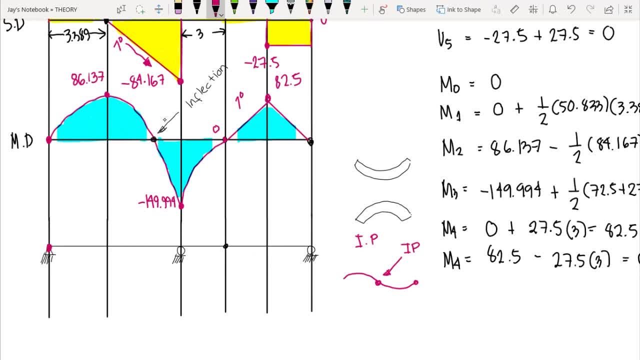 have a movement downward unless we have a settlement or soil settlement at that point. but take note, this problem does not state that there is a soil settlement at point a, so that means we do not have vertical displacement at this point. okay now, take note, at this point we have a positive moment, so that means we have a smiling curvature. 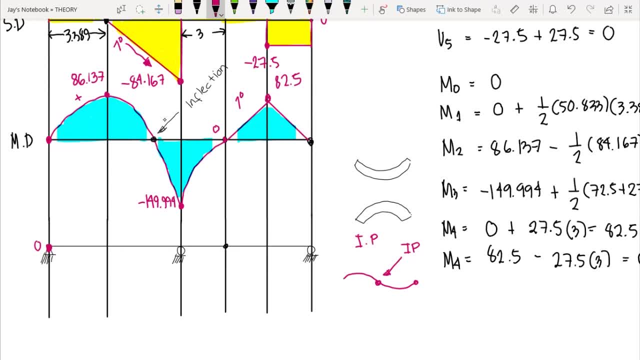 as our deflection diagram. so we have this deflection diagram. so this is our deflection diagram for this moment. but we should end at the inflection point. so again, this is the inflection point. so at that point there is a change in curvature, so from smiling it becomes frowning. 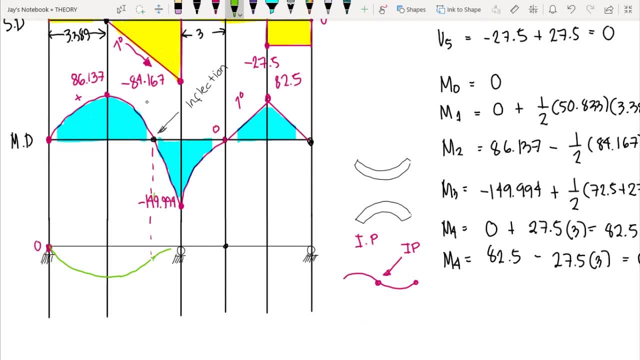 okay, so it becomes frowning. okay now, take note: since we have support at point b, that means our beam is restricted to move vertically at this point, okay. however, this is invalid if we have soil settlement at point b. okay, so we have to stay at this point. so now for this moment. diagram sox. 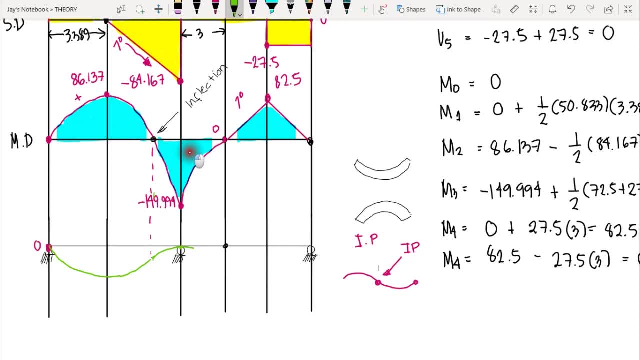 again, this is still negative moment. that means we have a frowning curvature for our deflection diagram. so we go here then. at this point, since this is internal hinge, at this point we do not have moment and our moment here is zero. that means this is the inflection point. okay, so this is the 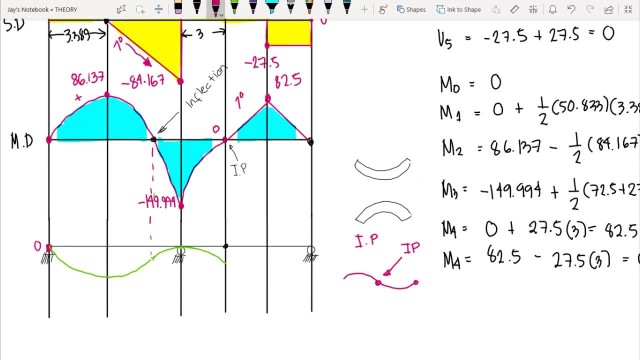 inflection point or the change in curvature. so we have, we have to change our curvature from concave downward to concave upward, since this one is a positive shear, or positive moment rather. so that means we have a smiling curvature for our deflection, and then, at this point, we still have 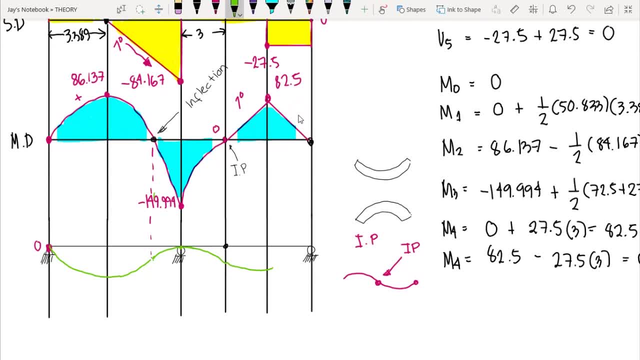 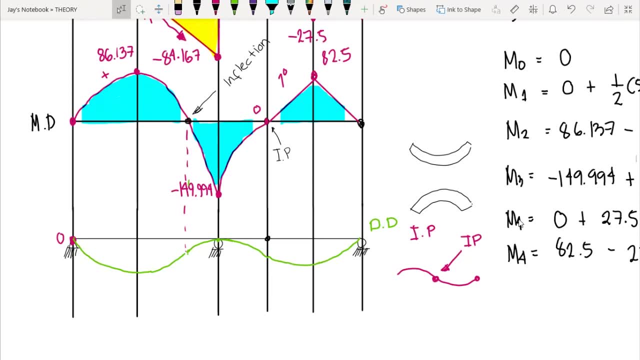 a positive moment. so that means we have- we still have- a smiling curvature. so at this point here. now take note this deflection diagram here. this is just an approximation, since we do not know yet, you know, the value of our deflection. okay, so unless if you know the value of our deflection, then we 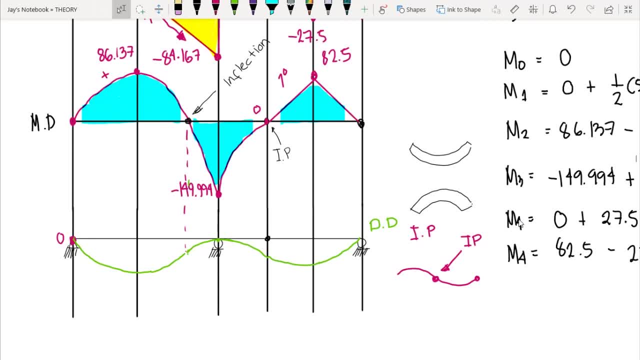 could possibly know the direction of our bending. okay, it could be upward or it could be downward. vertical deflection and, of course, we would also know its curvature by computing its slope, just like this one. we would have a slope here, like this one here, okay, and we would also have the slope at: 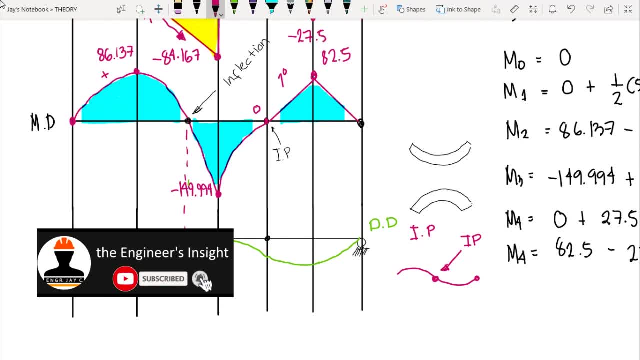 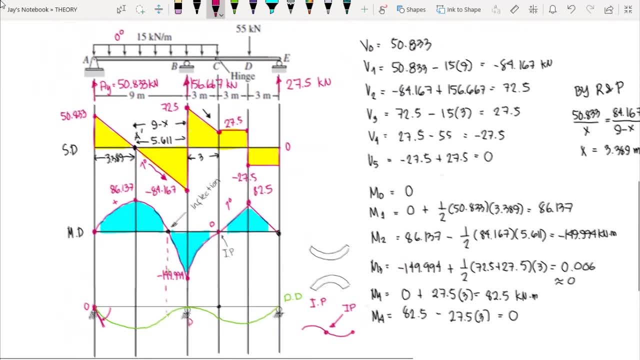 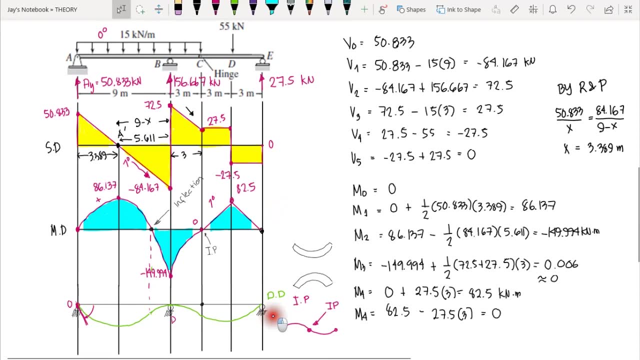 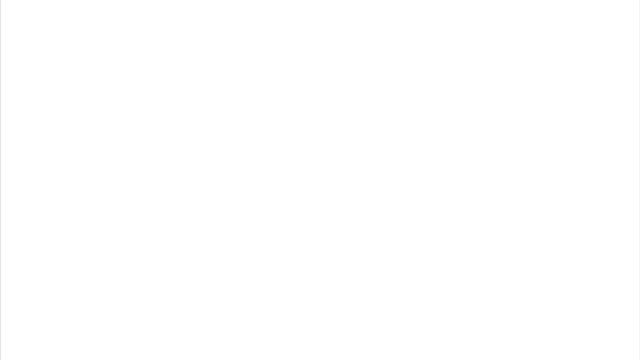 have a slope at point t. so by computing this we would have a slope at point t. so by computing